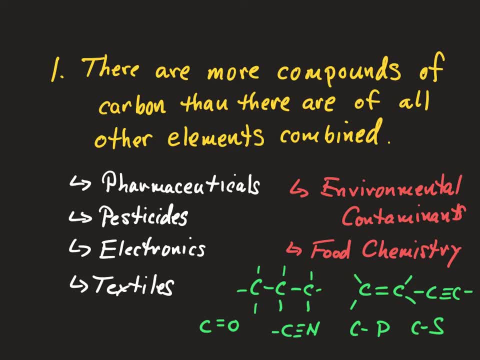 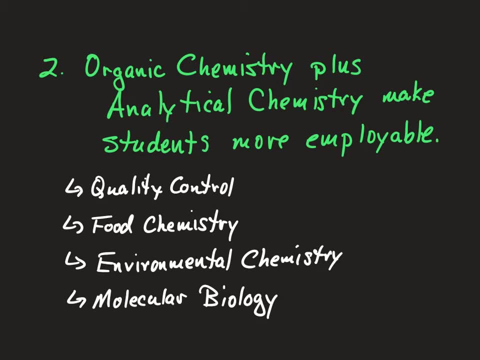 And that leads to its flexibility in terms of what we can make from it. If you consider the combination of organic chemistry and analytical chemistry, those two classes together make students more employable, right? Obviously, chemistry majors take these, But biology majors who take these, find that they have much greater flexibility in terms of job choice if they're moving into industry, right? 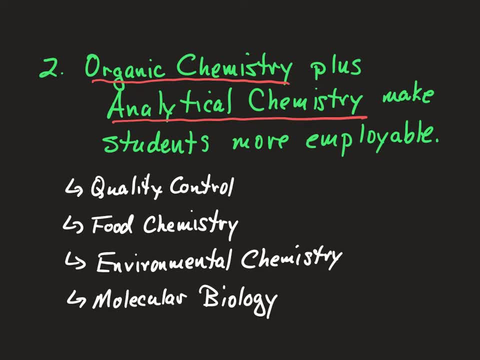 Areas like quality control, food chemistry, environmental chemistry, Even things like molecular biology. Techniques learned in analytical chemistry make students more employable, more productive and more knowledgeable. right So the combination of organic chemistry and analytical chemistry added to any other science area- biology. 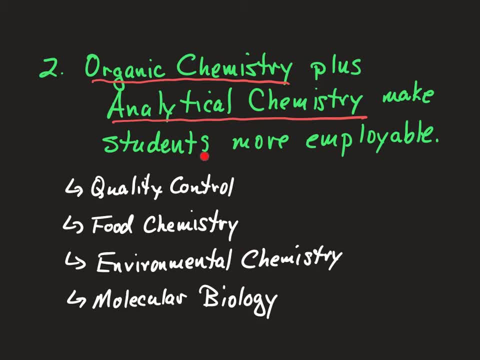 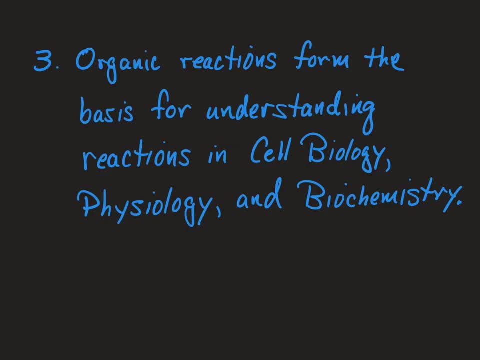 environmental chemistry makes students more employable in chemistry related fields. Another important point is that organic reactions form the basis for understanding reactions in cell biology, physiology and biochemistry, and so they form the foundation for study of most of the biomedical sciences. 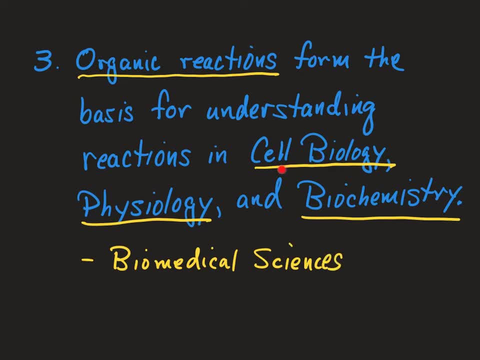 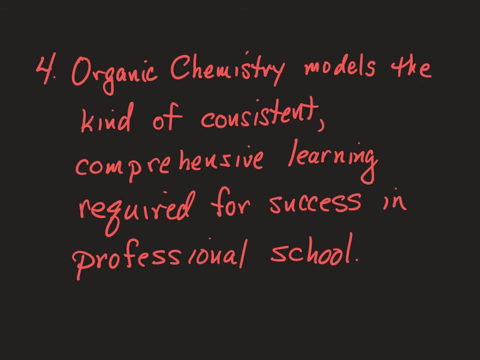 Right. All of these other areas study reactions of carbon-based compounds, and so anyone studying the biomedical sciences, organic chemistry is the foundation for that study, And for pre-professional students this is probably the most important part. Right, Organic chemistry Models the kind of consistent, comprehensive learning style required for success in professional school. 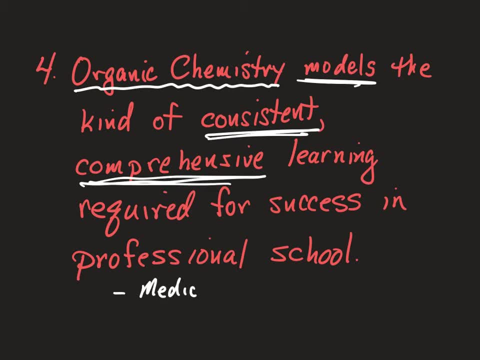 So again, if you're going into medicine, dentistry right, pharmacy, optometry right, we can probably name several other choices right. The way you learn in organic chemistry Is a measure of your ability to learn in a particular way.